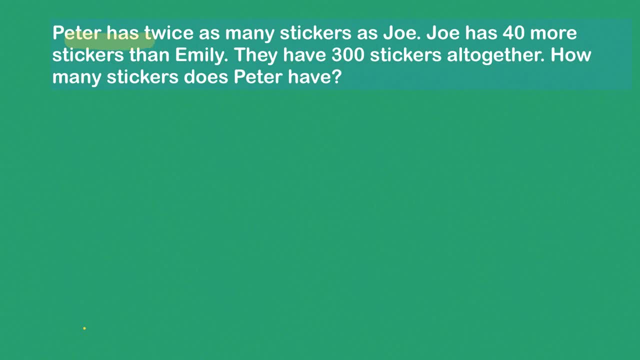 blocks here, and what I'm going to do is I'm going to draw my Peter block and I'm going to draw my Joe block, because it says here that I know that Peter has twice as many as Joe. okay, So what I'll do here, 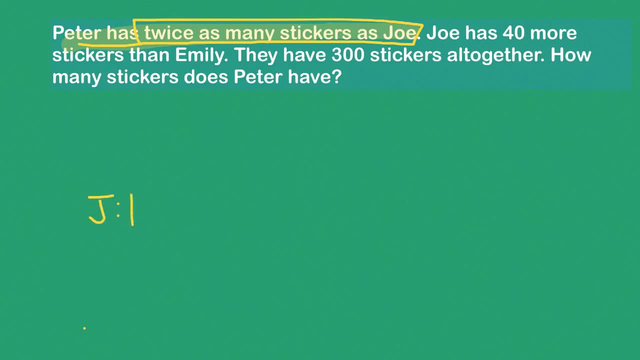 is. I'm going to draw my Joe block. There's Joe, And if Peter has twice as many stickers, well, he's got Joe a Joe block, same size, except he has that same block twice, right? He has twice as many. So far, so good, right? Okay, next thing I'm told is that Joe has 40 more than. 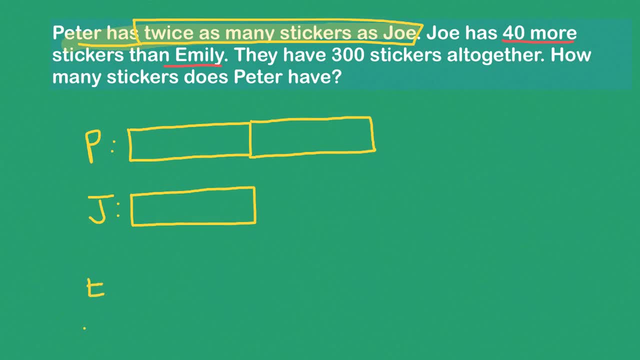 Emily. So Emily's got the fewest stickers. Joe has more than her. That means Emily's block is going to be shorter. right, It's smaller. Maybe I'll make it red to show it's not the same size. We have something here that shows it's shorter, correct So? and together they have 300.. 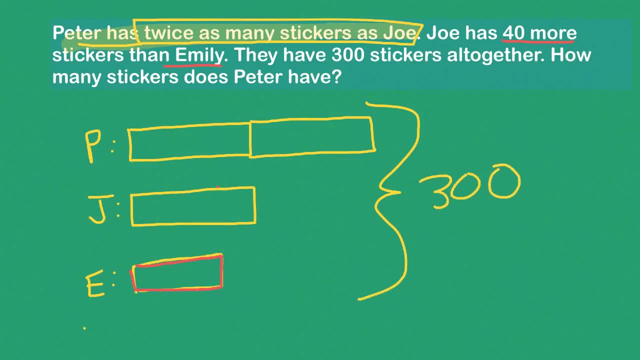 Now we have the same thing here and now we have the same thing here, And this side is going to be little。 Now, with the bar models, what we like to do is we like to divide to find one block. However, right now I cannot divide because I don't have even sized blocks. You can only divide when you're dividing things evenly, right or sharing evenly. These blocks are not the same size. I know that the Joe block is bigger than Emily's and each of Peter's blocks is also bigger than Emily's, so they're not the same size. 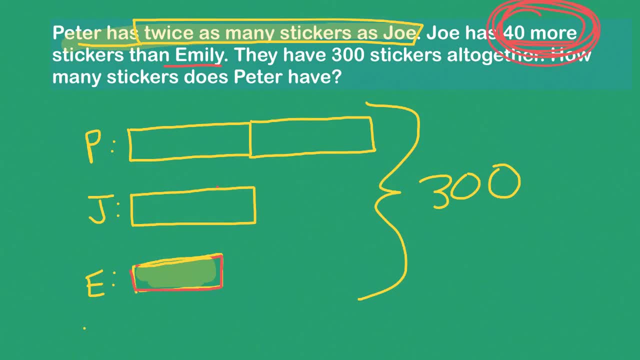 good thing is I know exactly how different they are. They're 40 different. That means I can take a little marker here and I can show that Joe has 40 more than Emily right there right Now. remember that Joe's block and Peter's block are identical, right These? 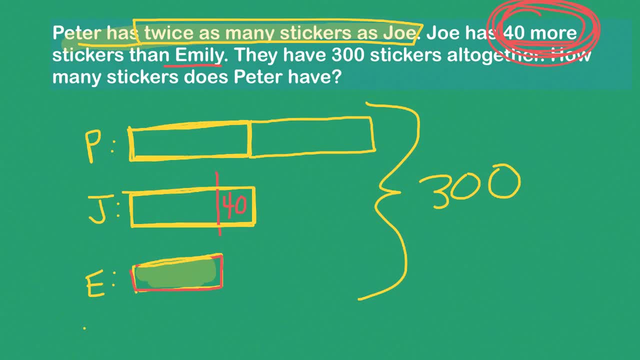 two are identical. That means where I drew a little 40 on Joe's, I can do the same thing on a Peter block because it's identical. This first Peter block is also identical to this block, so I can do that same thing there. Okay, so what do I notice? now Let's look. 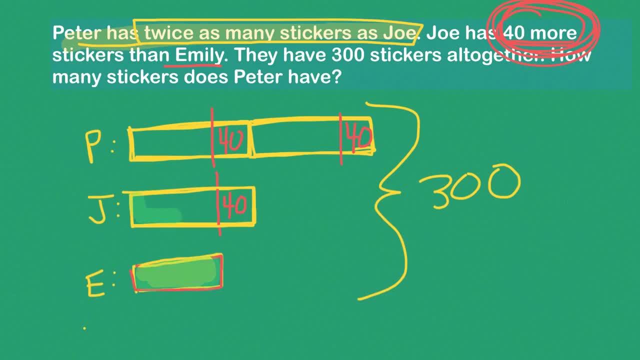 at this Emily block. Now I see, if I look at Emily's block, I now have a similar block for Peter and Joe, Right, Except Peter and Joe have little extra bits hanging off. If I get rid of those extra bits then I can divide by these: 1,, 2,, 3,, 4 equal size blocks. You see these little green. 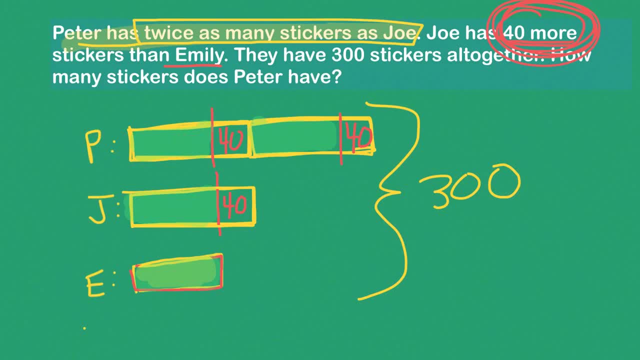 bits 1, 2,, 3, 4. They're the same size. So if I get rid of these extra 40s, then I can divide by 4. Well, what's the math For getting rid of things you subtract? Okay, so I see here that I've got 40 and 40. That. 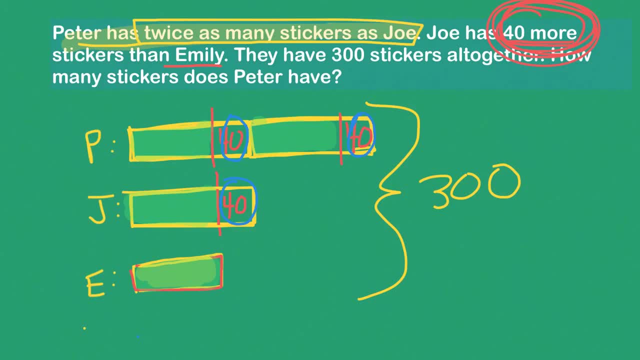 will make 80, and this 40 would make 120.. I want to get rid of those. Get rid of them is subtracting. Let's subtract 120.. If I do that, I get 180.. Now, remember, the 180 is: 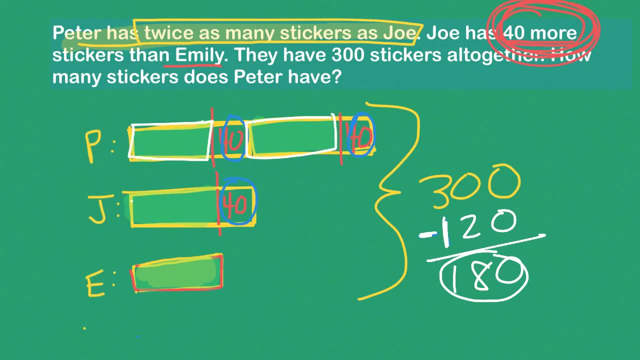 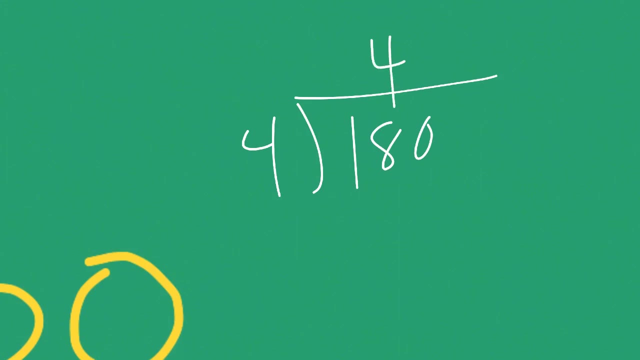 shared amongst these four blocks. That's all of these. It's not one block, It's all of these. So I can now divide 180 by 4.. 180 by 4.. You know that 4 and 4 is 16.. There's 2. 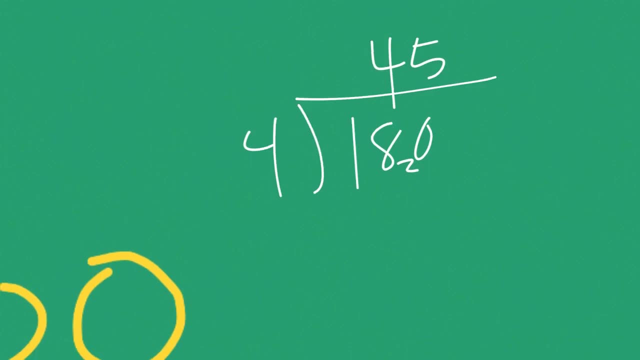 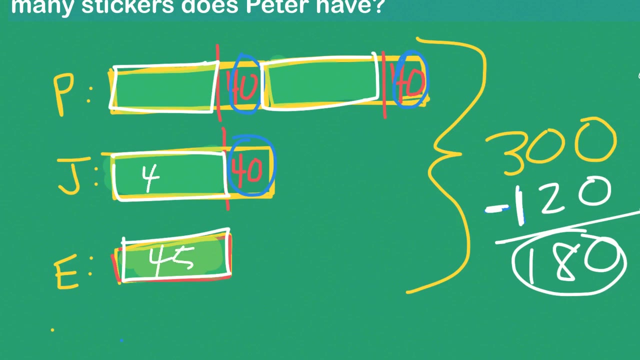 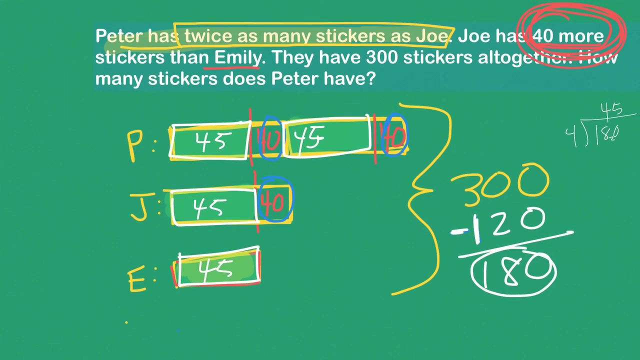 extra, and that's 4 into 20.. It's 5.. So 45.. So each of these blocks is 45, 45,, 45, 45.. Okay, and my question, remember, is asking me, Don't forget what it's asking you. It's asking us.